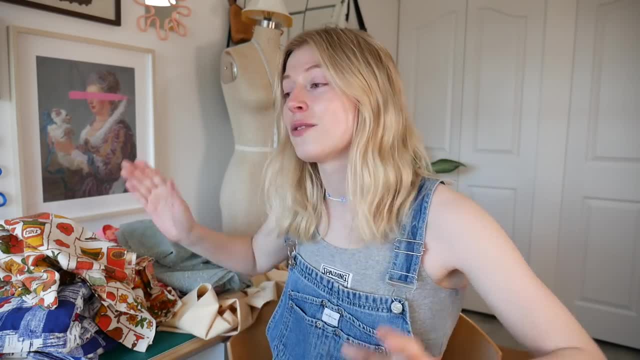 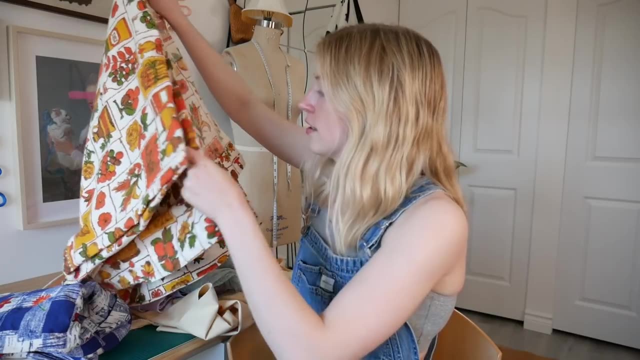 And also it's Earth Day tomorrow. So I recommend if you guys want to make a dress, try out your local thrift store First and see if there's any fun thrifted fabric there. If not, try the curtain section- This, legit, is a curtain right here- or the blanket section. the blanket section. 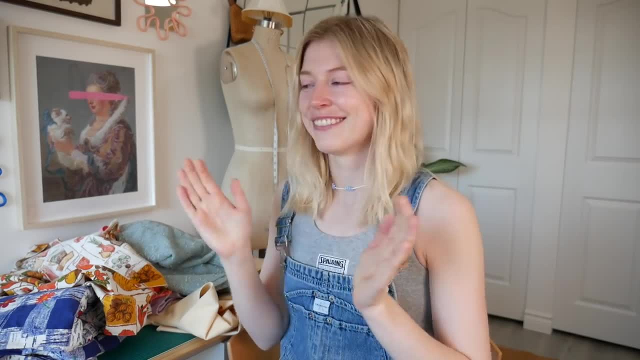 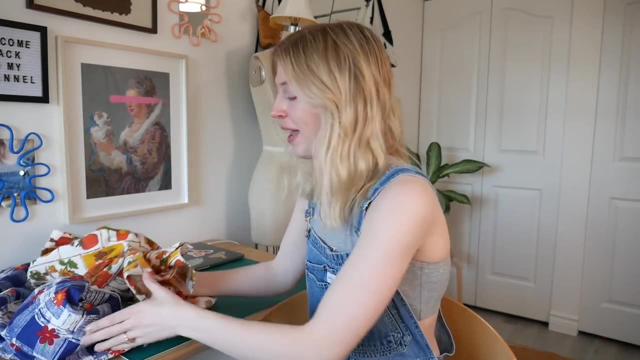 I have found some good fabrics there as well, But other than that, we can get started. We can get started. I got to pick my fabric first, because I got a lot here. I got a lot of thrifted fabric here. I decided we're going all out today and we're using these two fabrics. 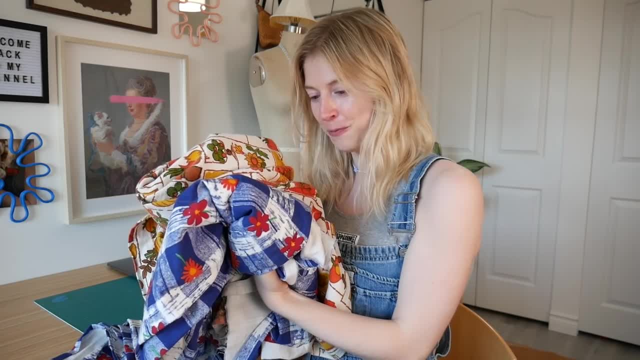 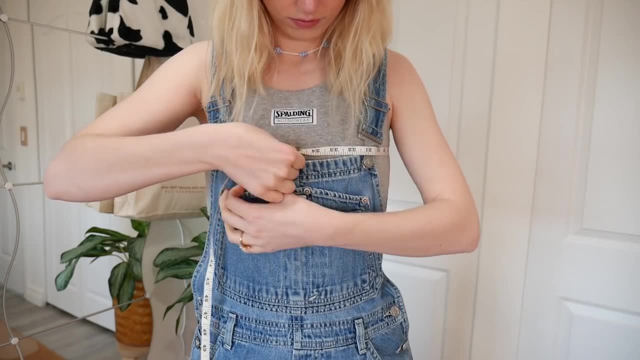 I'm low key, super scared, but also really, really excited to see how it turns out. So we're going to need two measurements in order To get the top. So the first one you're going to need is your bust. It doesn't have to be your exact bust. 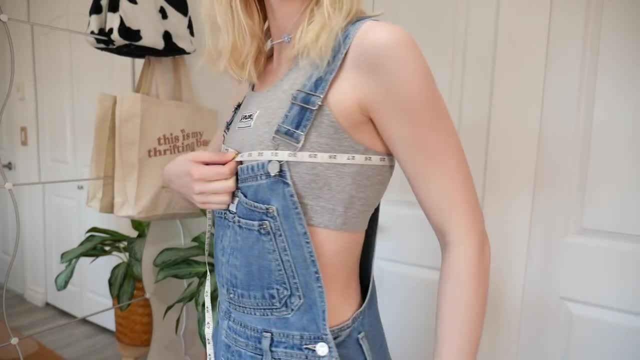 It can be a little bit bigger just because this is going to be a nice flowy dress. So I just did it over top of my clothes. You don't have to be super exact, And then the next one you have to get is how long you want the top to be. 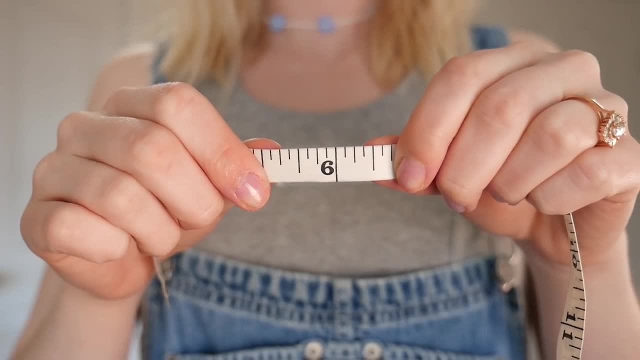 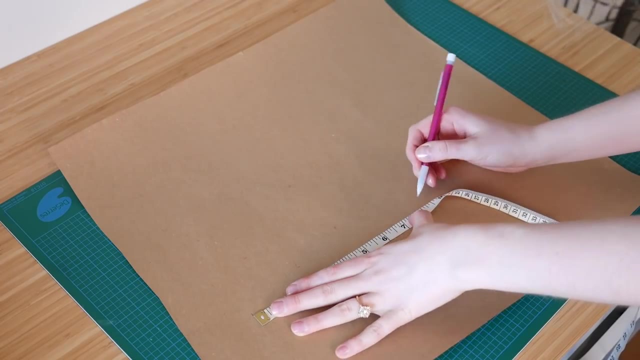 I didn't want it to be too long, so I measured it to be about six inches. So now we're going to make the pattern, You're going to take your bust, You're going to divide it by four in order to get the width of the pattern. 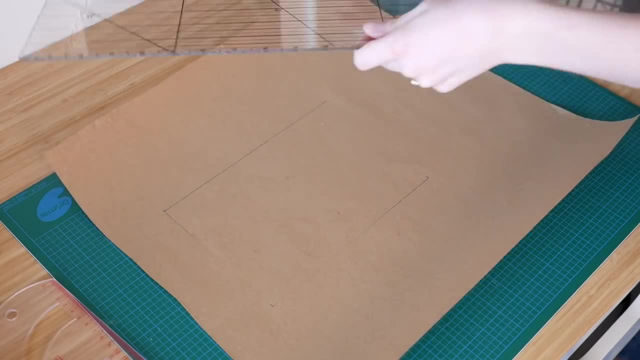 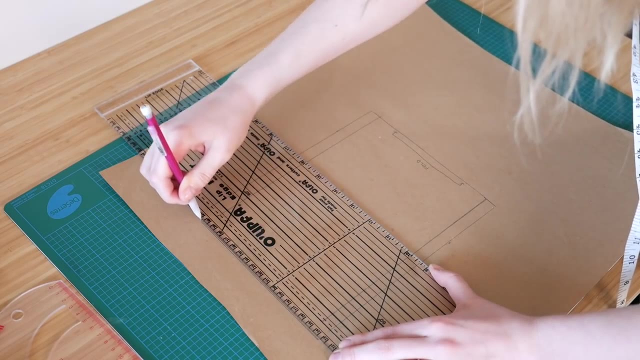 And then you're going to take the height of what you want for the top- So mine was six inches- And then draw a rectangle with those two measurements. One of the short sides is going to be placed on the fold, So I wrote down fold, so I wouldn't add the seam allowance. 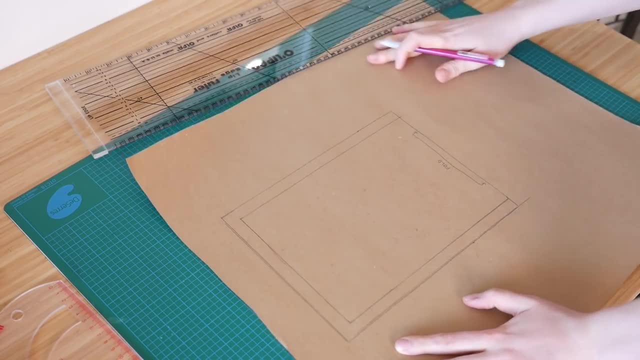 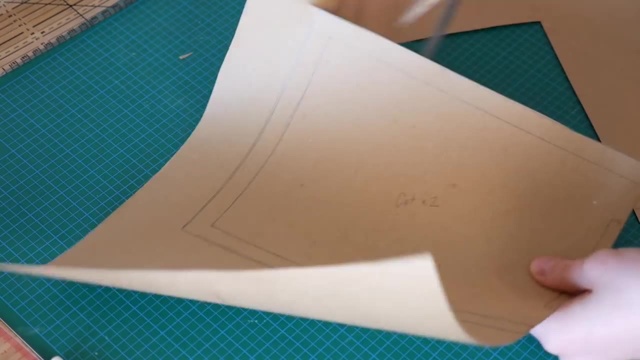 And then I added the correct seam allowance to the other three sides. In my case, I added a half inch seam allowance And after that I just cut it out and we're done the pattern. It's pretty simple. All we're doing is just making a nice rectangle. 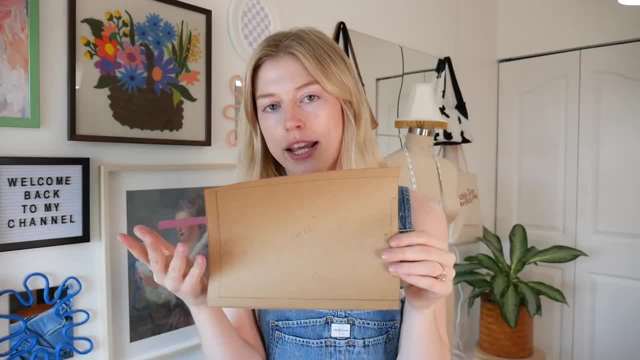 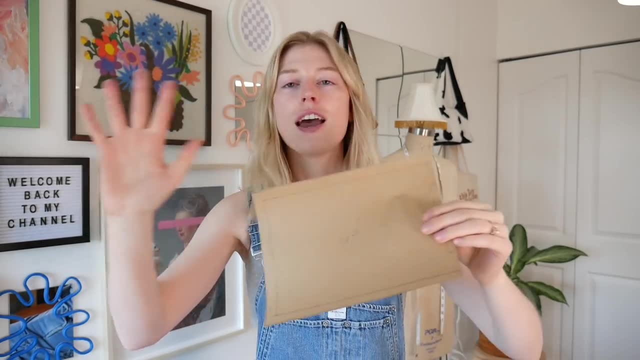 So I have my pattern done. It is just a rectangle, It's super simple, but I like making a pattern, just so I don't forget anything. The seam allowance is all. They're the correct measurements. Everything's everything's just there. 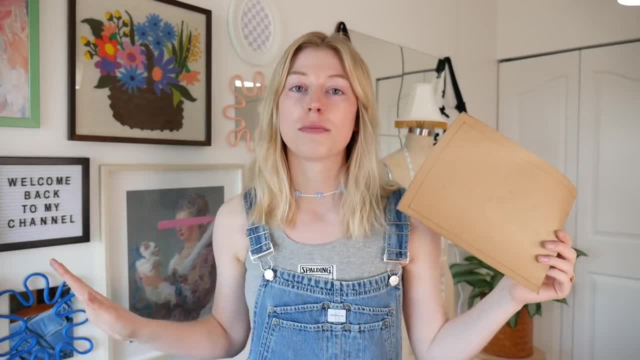 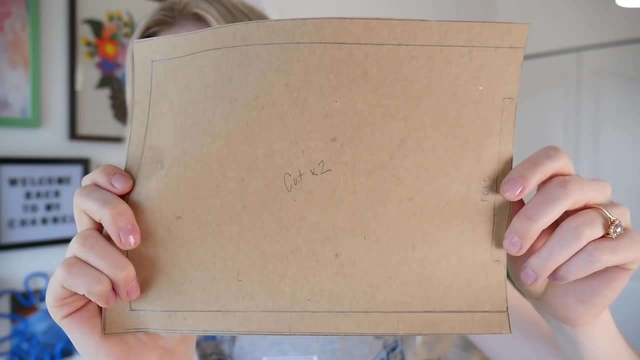 So I made this pattern. This is the only pattern we're going to make. Everything else is just going to be cut right from the fabric. So, don't worry, won't make you do any more math, or can't guarantee that yet, But this is what my pattern looks like. 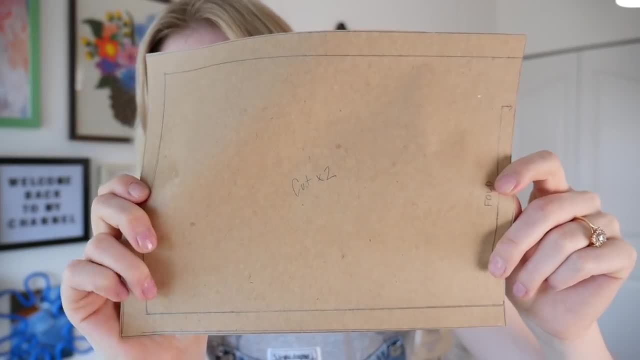 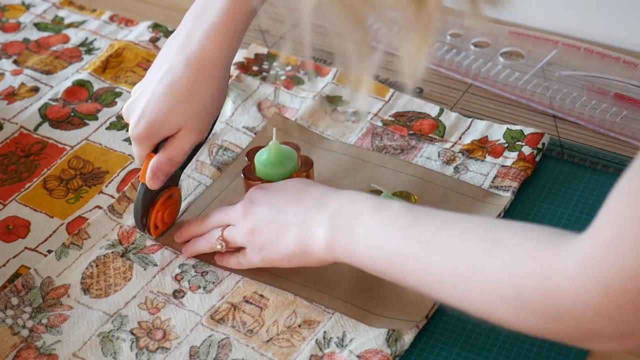 And I'm going to cut this on the fold here, So I marked that, so I don't forget. And then, of course, seam allowance on the all the way around, So let's go ahead and cut it. So my first unprofessional tip of the day is: if you don't want to actually 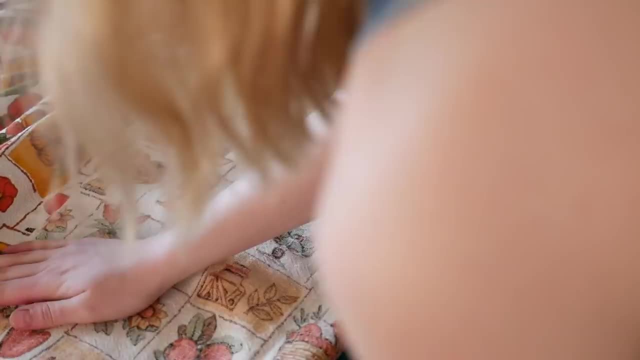 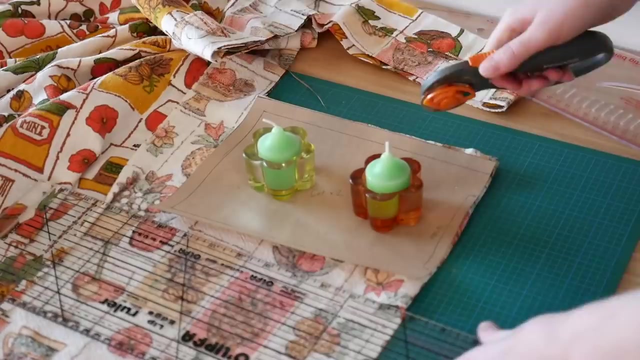 bring the pattern to the fabric. just get some candle holders and put it down over top. It'll hold it down, It won't move, but I'm just cutting it out. I ended up cutting out four pieces of this because I'm using two for the outside. 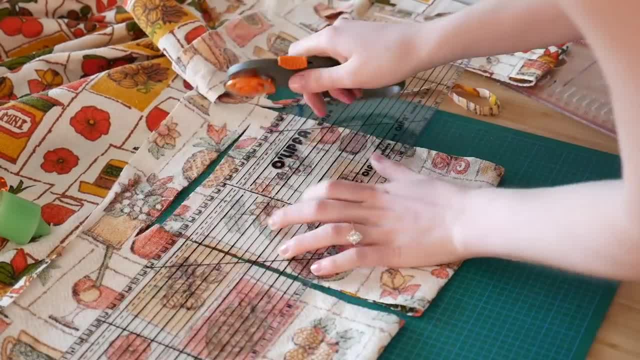 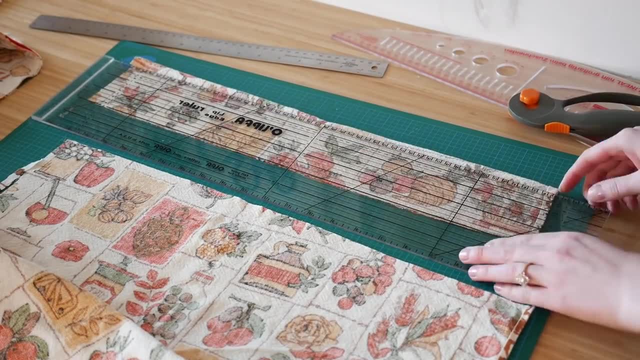 of the dress and I'm using the same fabric for the lining. So that's why I cut out four. And then I started cutting some straps that were three inches to four inches wide, And then I ended up cutting four pieces of those. So you should have four pieces like this for the top, two for the liner. 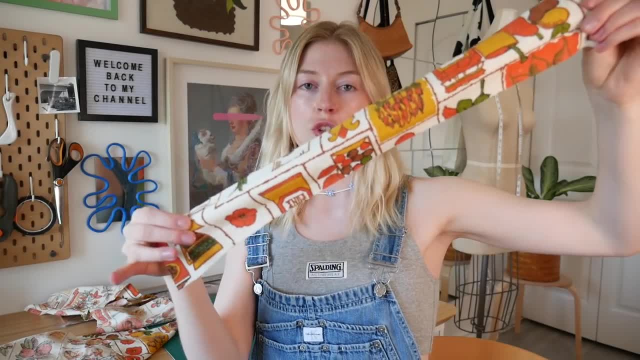 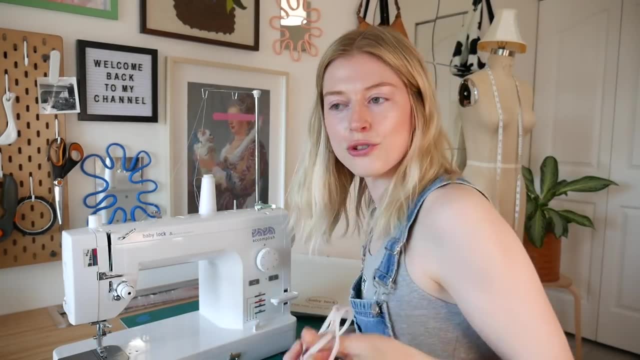 two for the outside of the dress, And then you should also have four straps, you know, two for the front and two for the back. I'm lazy, So I'm just going to keep my white string- or technically it's thread- on my machine. 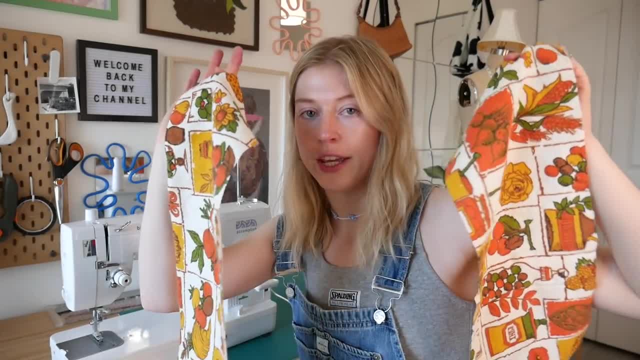 Yeah, we're just going to keep white on it. So the first thing you're going to do is you're going to take two of your pieces, You're going to put right sides together, And then you also want to make sure that the pattern is facing upright on. 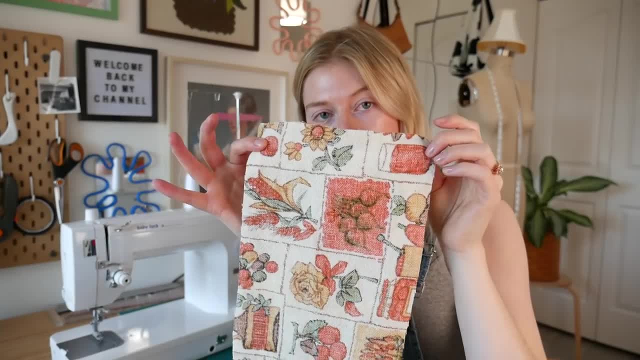 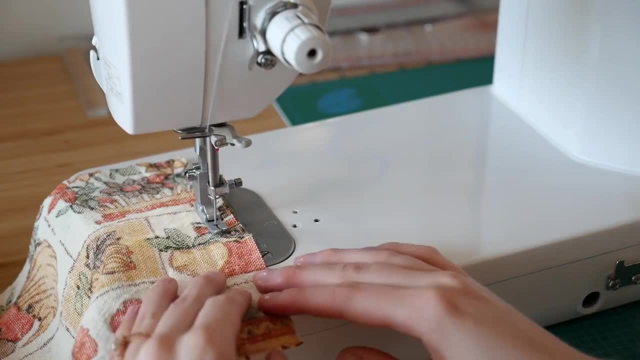 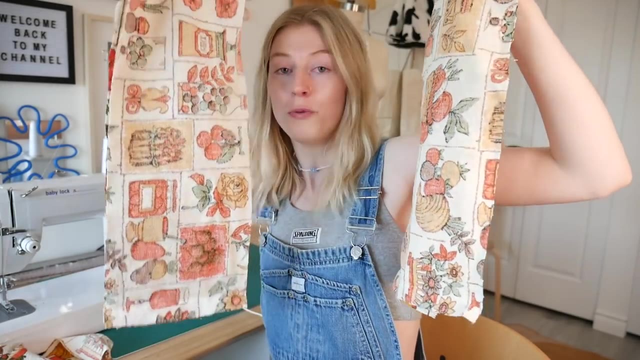 both sides And we're just going to do a straight stitch along this side, right here. So now that we have our two pieces of fabric looking like this- So it was four, but now it's two pieces- Now they both should look like this: two very long pieces of fabric. 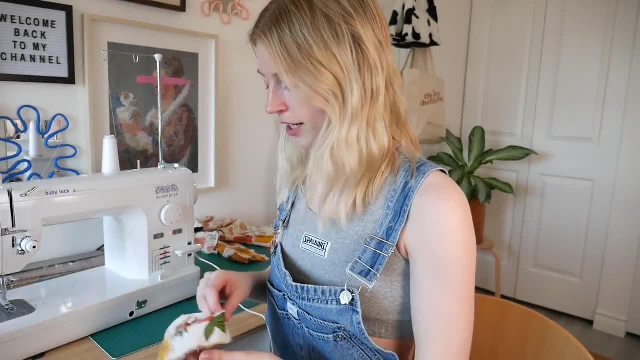 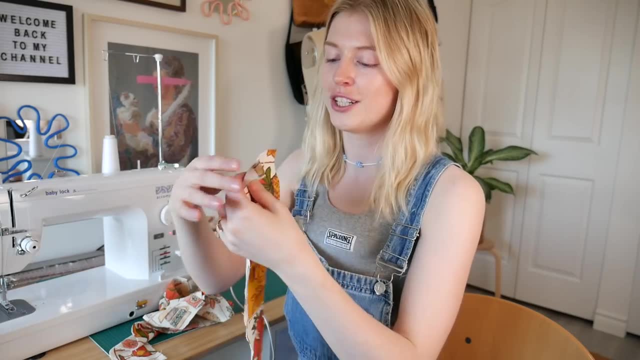 But once we have that, we can just throw it on the side, because we don't need that right now. What we need is we need our straps. I almost forgot the name of it. We need our straps here. So what we're going to do with our straps is we're going to fold it like a. 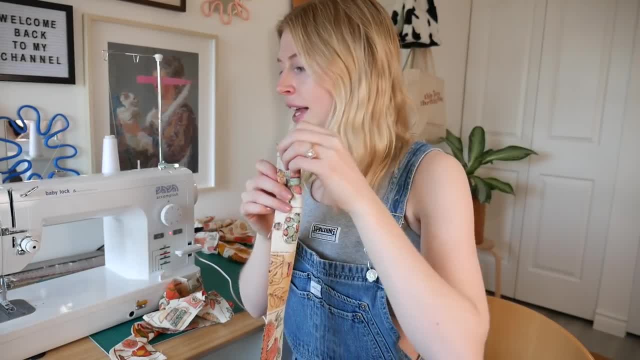 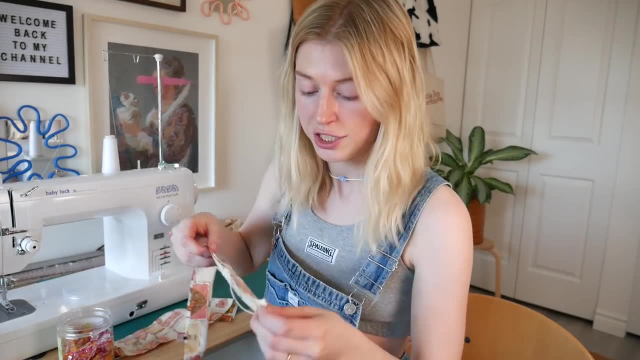 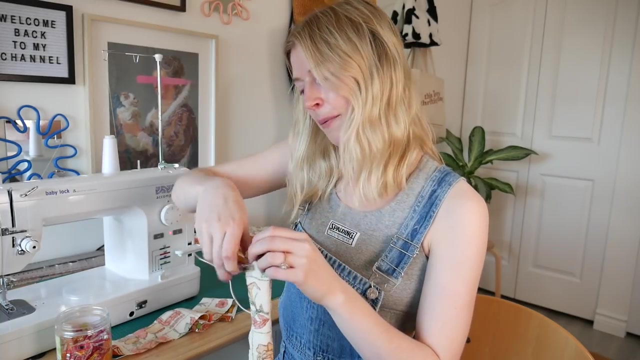 hot dog bun, not a hamburger hot dog bun. We are going to pin them or clip them with the right sides together. Typically, I actually don't pin this, but because I'm trying to teach you guys get habits, I'm going to pin it today. takes a little bit more time, but it's worth it. 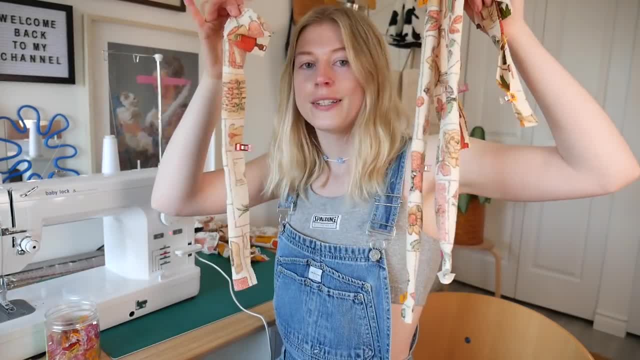 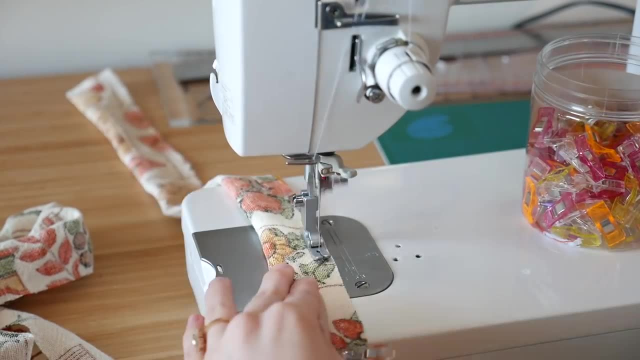 because then you don't mess it up. Okay, Now we need to sew them. So for sewing these straps, I am just doing a straight stitch at the top of one end, before I go ahead and do a straight stitch down On the whole side, just because I want one end to be nice and finished. 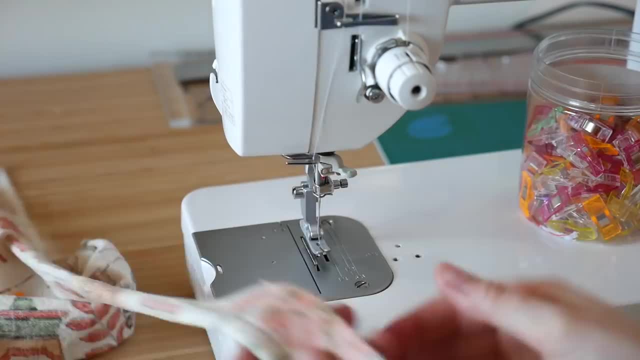 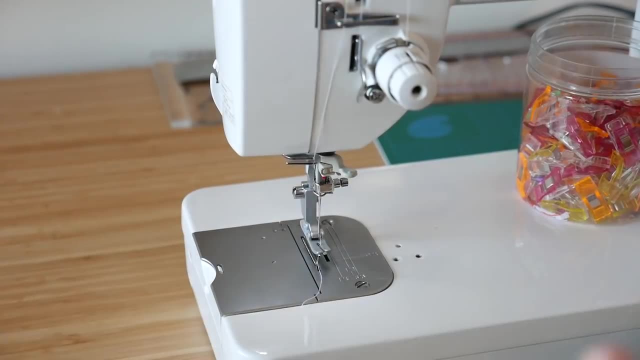 because we're going to be tying the straps together at the top, So that is why I'm doing like that. The other end is fine, open, because we need to switch them right side out, So we need that open. but I just did that for all four straps. 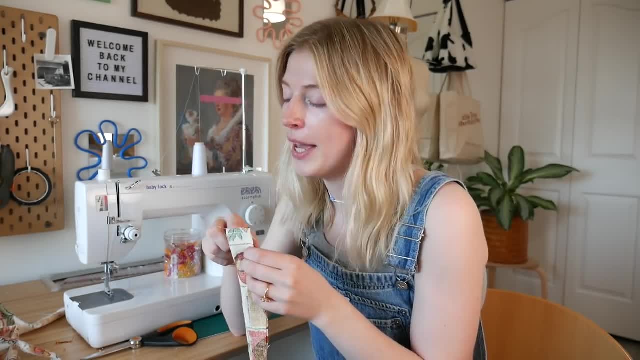 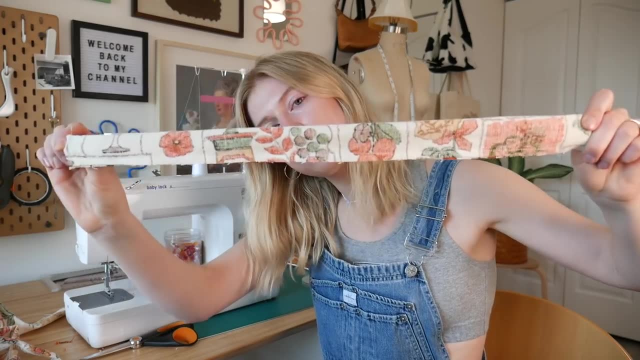 So if you guys watch my sewing video when I made my wedding dress, you would know I hate turning straps right side out, but these ones are okay because these ones are pretty thick, So it's gonna be kind of easy. So what I'm using here is I'm just using a safety pin and I'm taking the 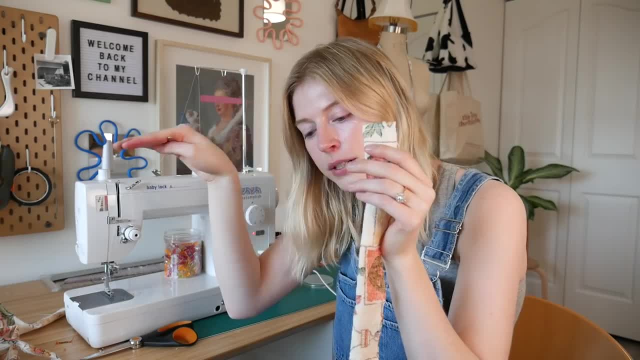 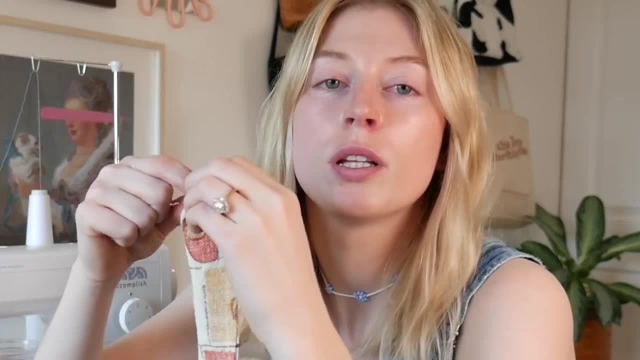 end where I did my little, my seam stitching at the top, and I am just going to make a little pouch, little pouch for a little kangaroo or a little safety pin. Then once I have my little pouch like that, I just put my safety pin in. 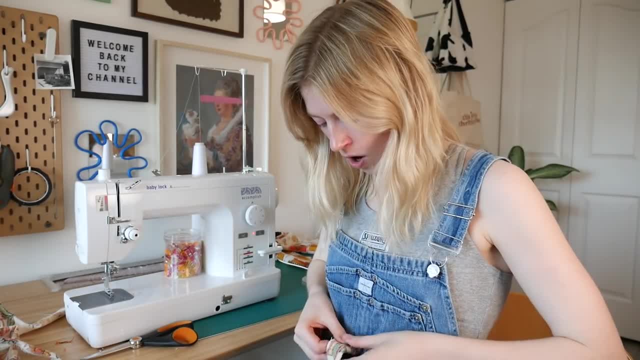 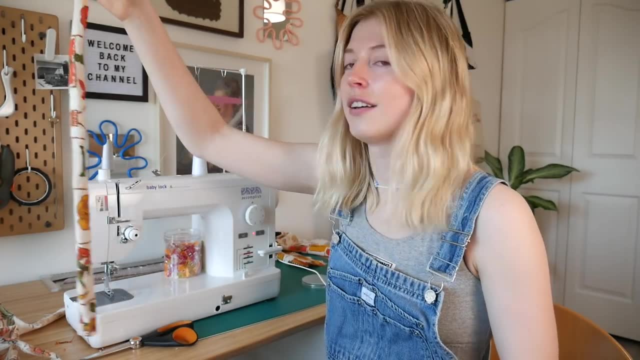 there and then we can try to push the safety pin all the way to the other end. Does that make sense? Makes sense in my head. favorite part: Isn't that beautiful? We have our first strap, So we have our four straps done now. 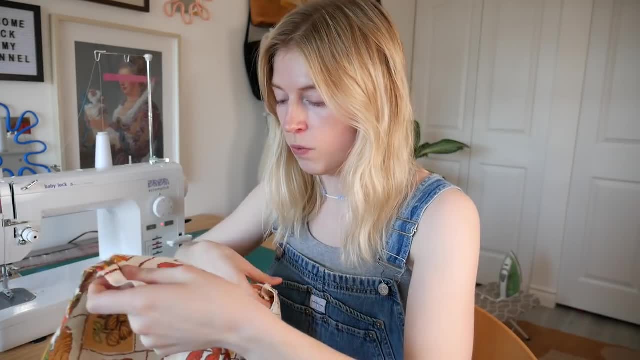 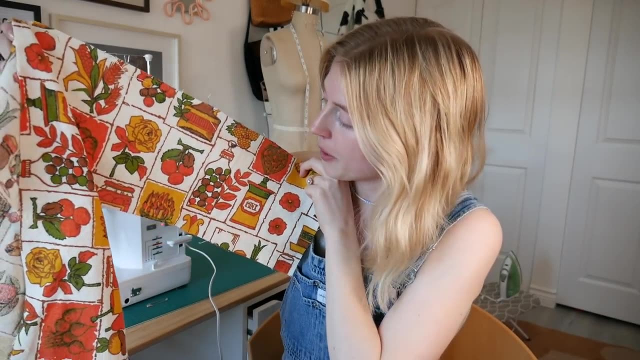 So now we can move on to actually sewing the whole top together. So what I'm going to do is I'm going to first of all make sure my fabric is the right way, that they're both facing the right way, and they are, they are. you're going to go ahead and you're going to pin the two seams together. 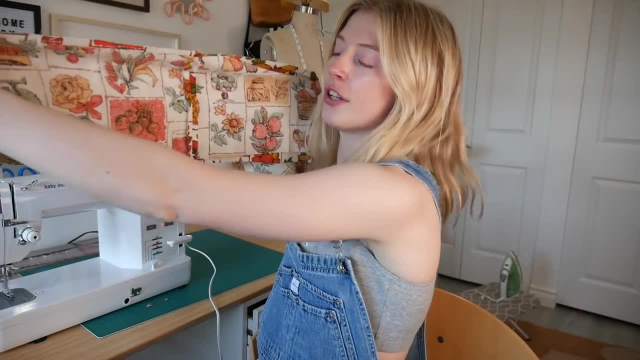 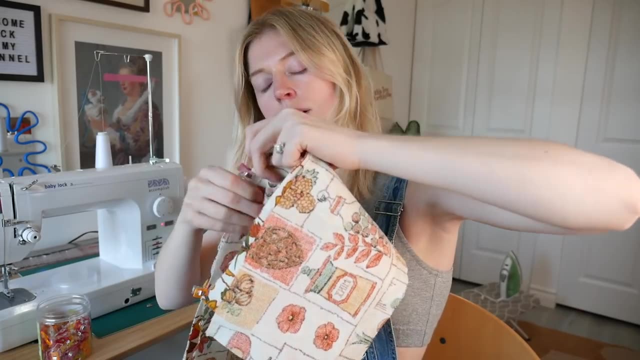 and you're also going to make sure that the fabric is right side together. So it looks like this and I'm going to take my clips here and I'm just going to clip the whole top of the top together: Bam, Bam, turkey and chicken. 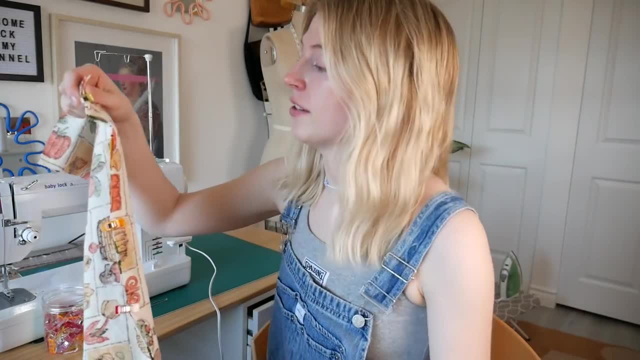 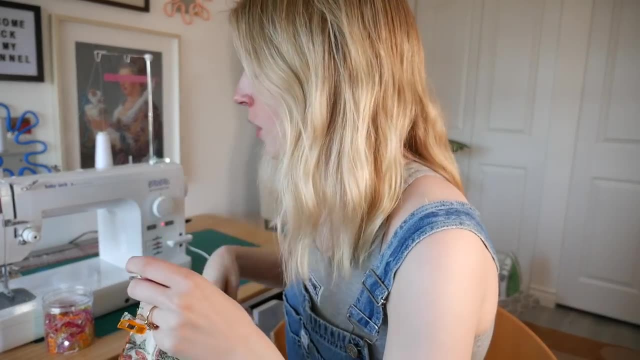 It is that or it's not completely done. We have it pinned, So now that it should look like this, your top should look like this. I could have showed you this on the table, But oh well, it's probably easier to show you on the table now, though. 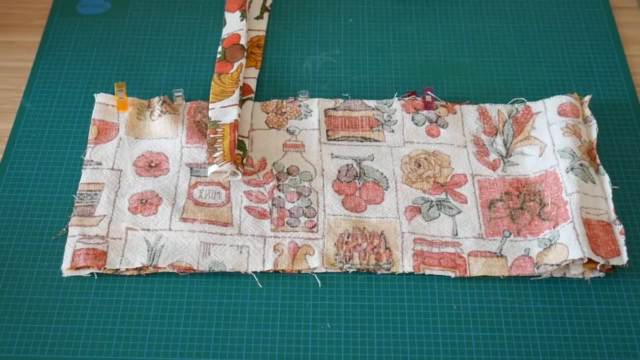 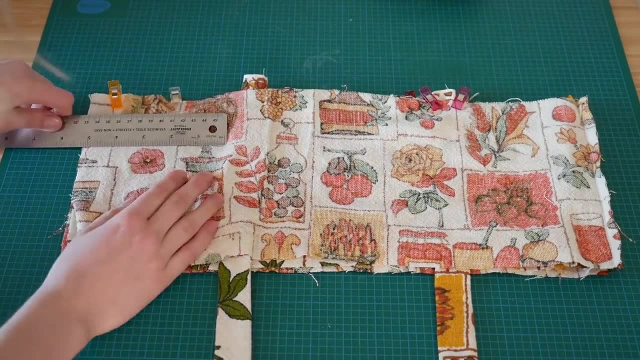 Okay, So the next step is we just have to line the straps up inside the top So you kind of open it up for the front and you go ahead and you can pin one strap and then you can open it up and pin the other. 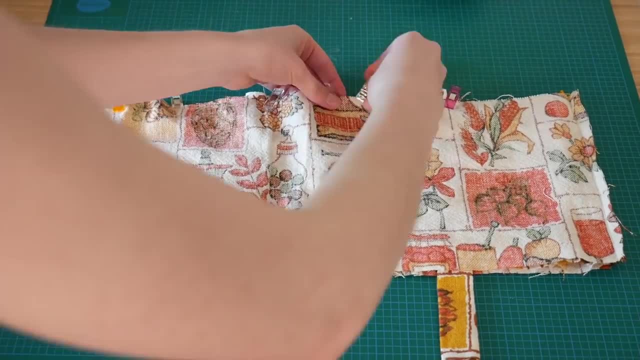 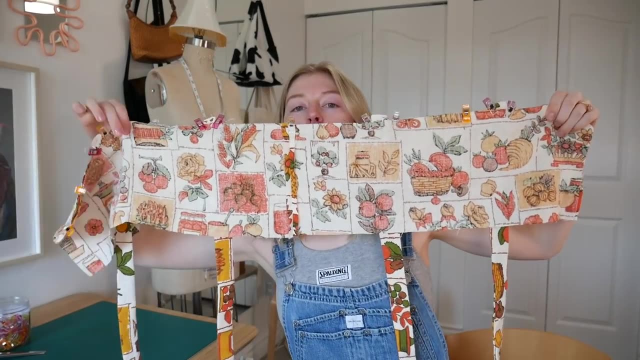 Strap for the front. Yes, I even got my ruler out because I wanted it to be perfect, So I did that, and then I just copied the same thing on the back. This is what my top looks like now, And once it looks like this- your top, we can start sewing. 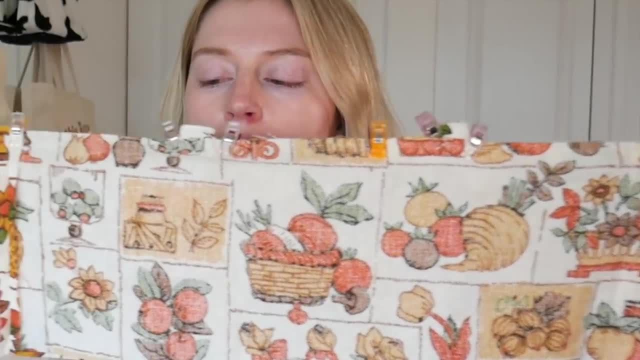 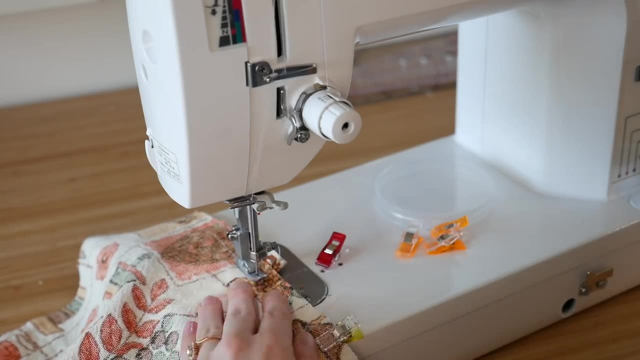 So I'm just going to sew along the whole top here. Just follow my nose right there. That's what we're going to sell from one end to the other. So you're just doing a straight stitch along the whole top and yeah, you just. 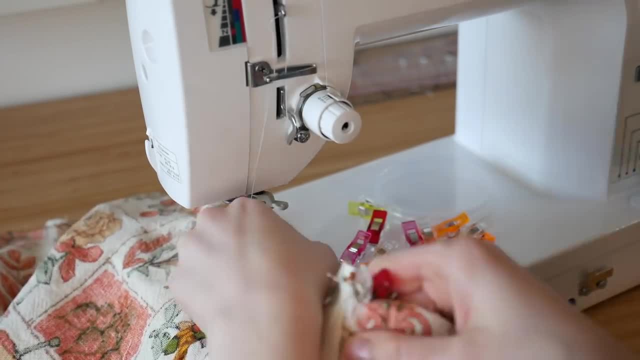 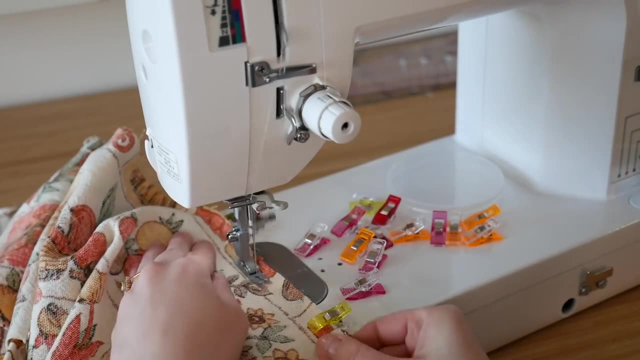 do it from one end to the other. It's nothing, Nothing special, Just do a straight stitch. And also I have a crack in my nose. still It sucks because I had to put Vaseline on it 24-7.. Like I'm constantly having to put Vaseline on my nose. 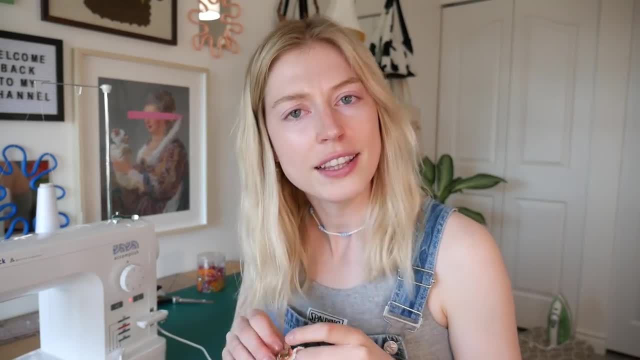 Benson, legit, just licked my toes the whole time. I just sewed that and he licked the foot that was on the pedal So I couldn't do anything. Okay, I guess I could have stopped and told them to, but I was filming for you guys. 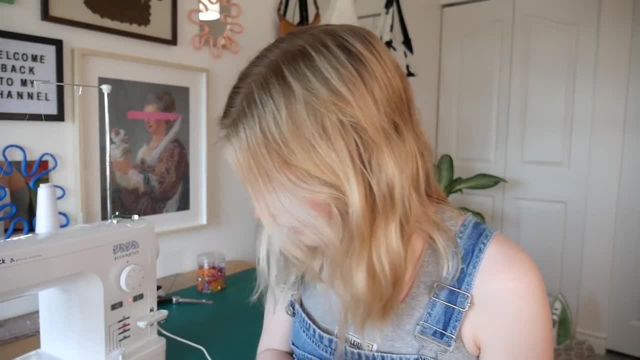 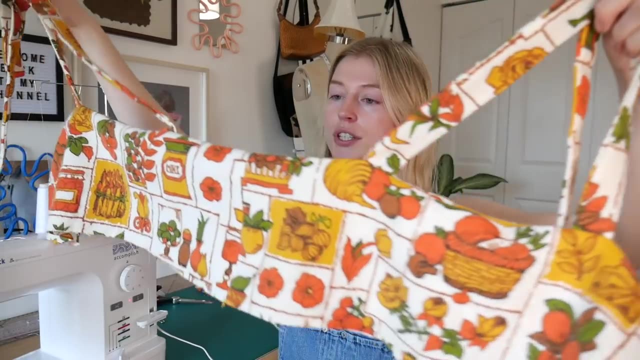 So I didn't want to stop. Anyways, other than my my toes being all clean now. Thanks, Benson. This is what the top looks like so far- Finally starting to look like a top. So I'm just going to Go ahead and iron the top of this and then we can do a top stitch. 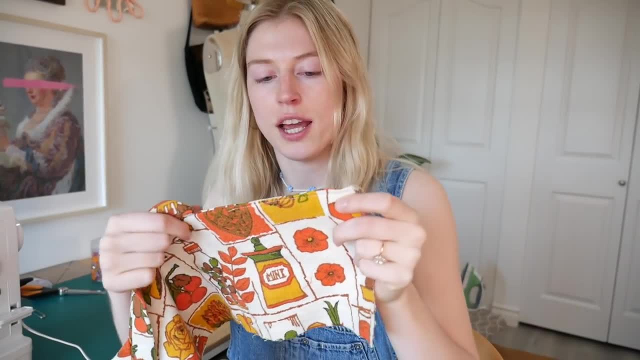 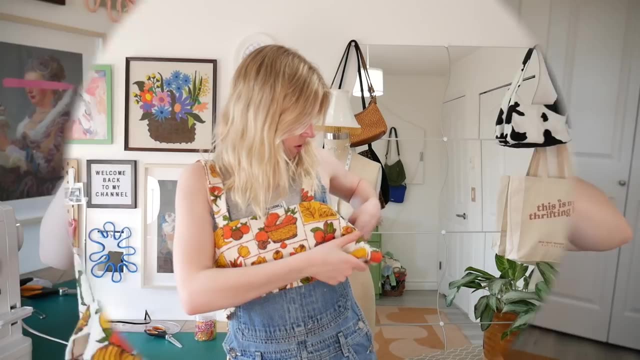 I just started doing a top stitch right here and I just stopped after a few inches because I don't think I like it. I kind of want to just leave it without a top stitch. So I'm just placing this top on and I'm not a huge fan of the placement. 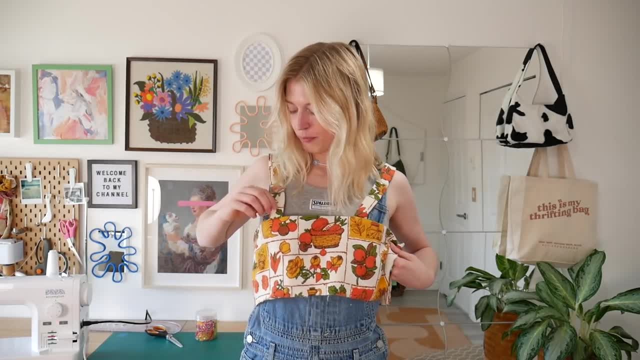 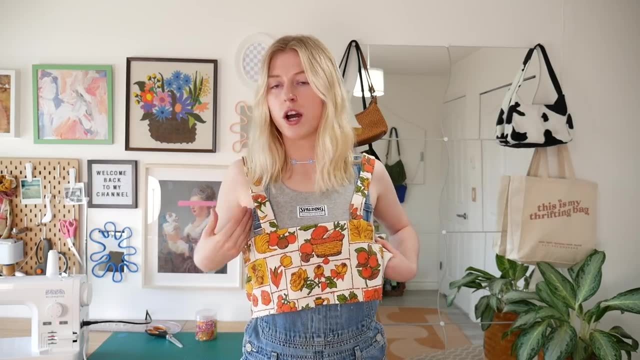 of these straps kind of looks like an apron. I'm going to seam, rip the front two straps here and I'm just going to move it out a little bit to the sides, just a little bit like an inch and a half, two inches Over on each one, and then I'm just going to keep the back to the same. 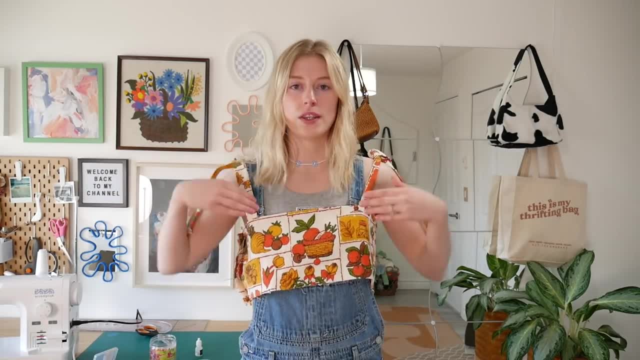 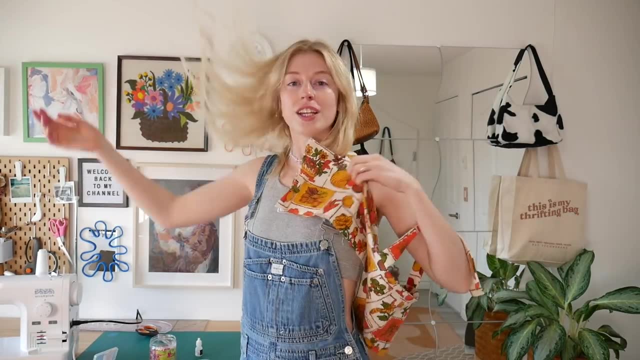 Okay, this is a lot better. This is a lot better. I ended up just moving them one inch outwards- the straps- and looks good. now, Now that we have our top all ready to go, we can do the skirt. now, Do I hit that note? 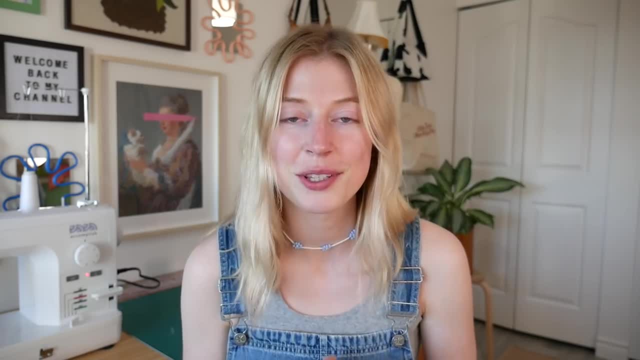 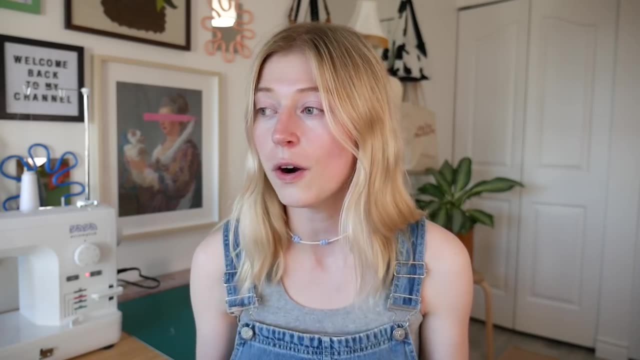 So we actually have a sponsor for today's video, which I'm so excited to share with you guys. Today's video sponsor is True Earth. I absolutely love True Earth and have been using them for almost a year now- Almost a year now. 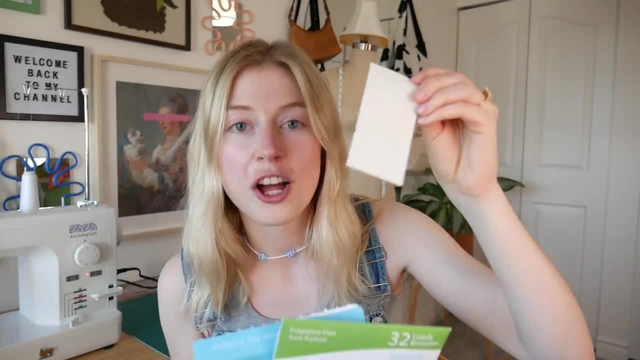 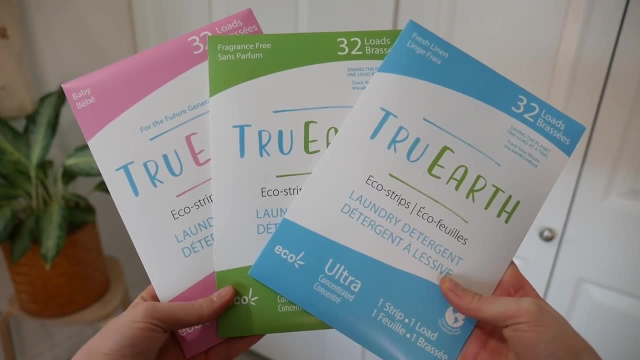 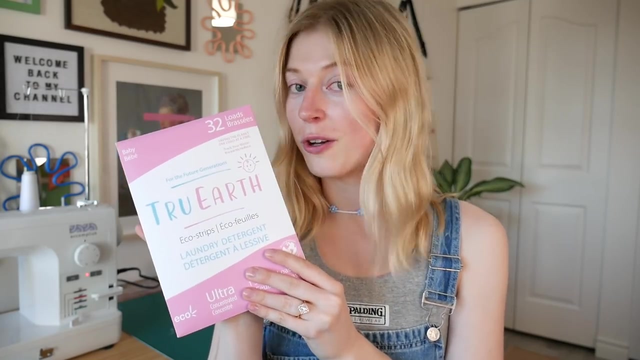 I've been using their eco strips. Here they are. They are laundry detergent strips. Isn't that incredible? This is for one load of laundry. pretty crazy, right? They have three different types. They have their fragrance free, They have fresh linen and, lastly, they have their baby formula, which is 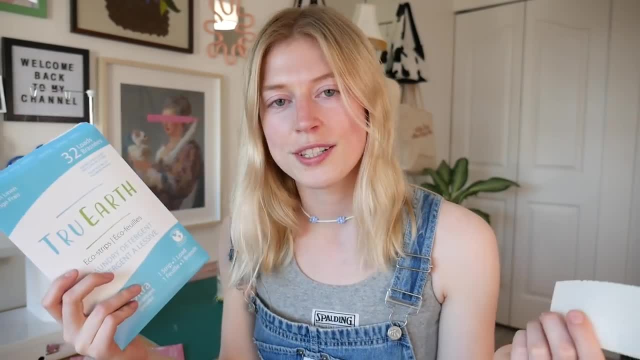 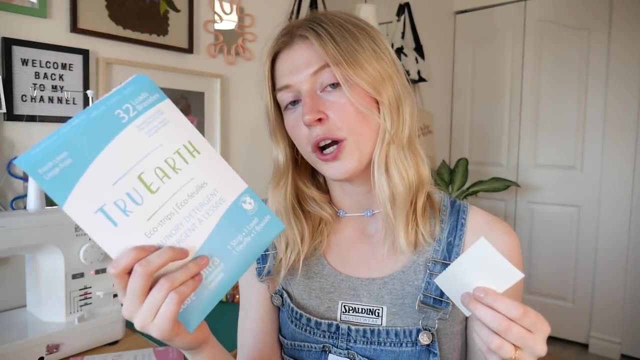 also fragrance free. My favorite thing about these eco strips is, of course, that there's no huge plastic container that you have to buy when you buy your laundry detergent. It comes in biodegradable cardboard, So that means you can just go and recycle. 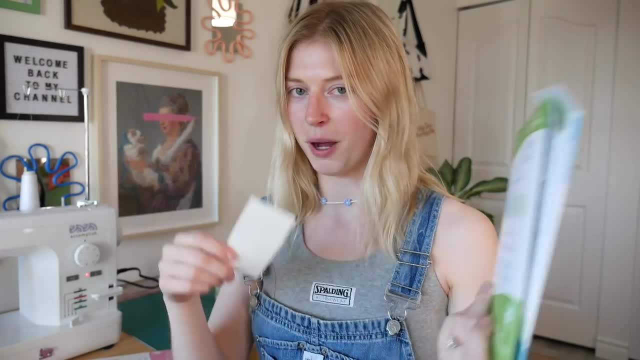 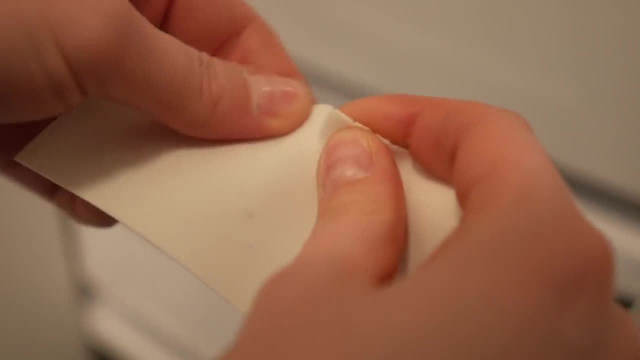 This after, or you can also biodegrade. it might be a little confusing. You're probably like: how do you use this? Like how does that clean your clothes if it's not liquid? Well, let me show you guys. So these detergent strips are just like your normal detergent, except you. 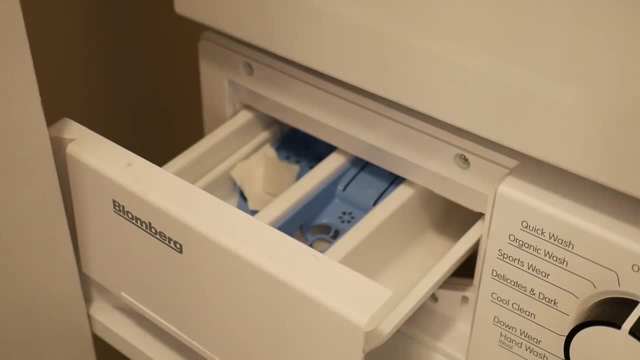 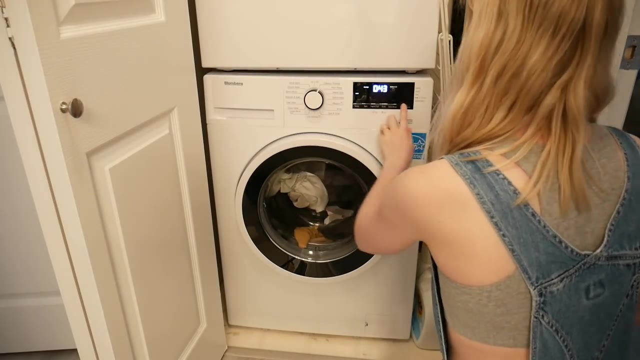 just have to tear it up a few times if you're putting into a detergent slot, but if you have a front-facing washer, you just throw it in, but that's it. They are the exact same washes. one load of laundry, just one strip and 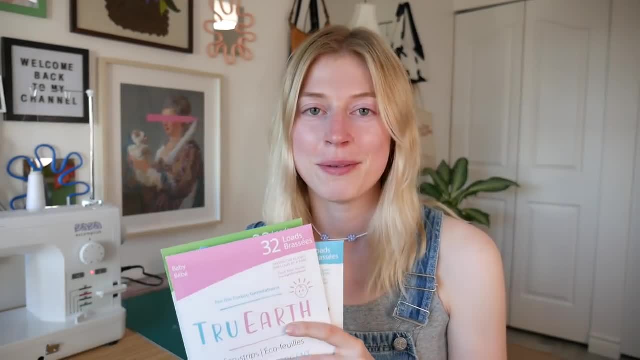 you're good to go leaves your clothes nice and clean. I was so happy I was able to partner with True Earth for today, Today's video. if you guys do want to try out their eco strips, I do have a coupon code for you guys. 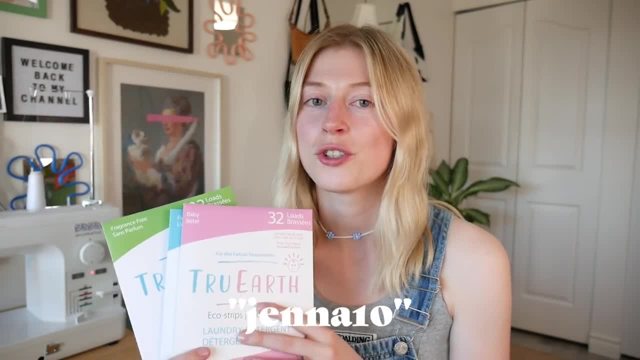 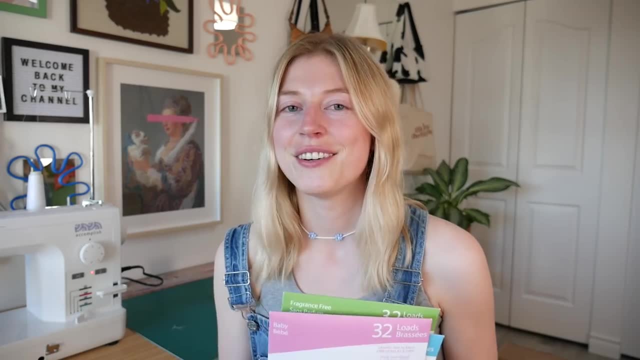 The coupon code is Jenna10 and you can enter that at checkout if you go to TrueEarthcom, or you can click the link down below in the description. Thank you so much to True Earth for sponsoring today's video, and let's get back to the sewing. 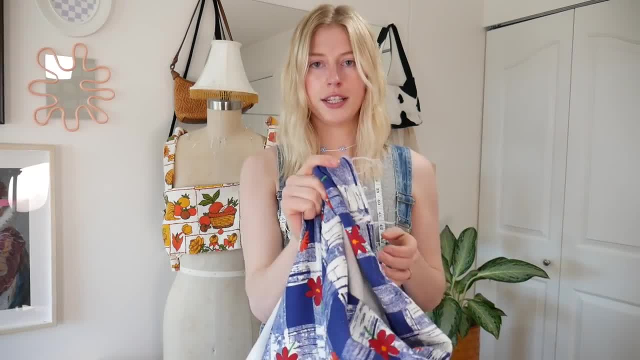 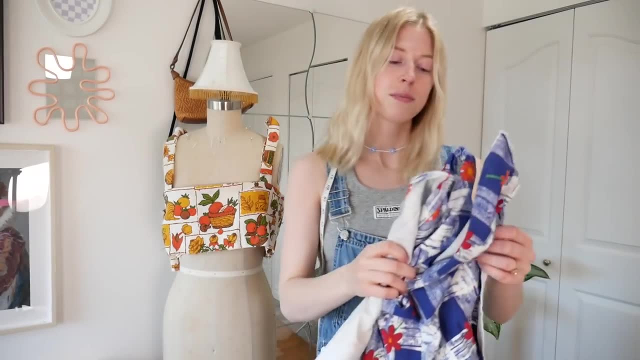 So to figure out how much fabric you need for your skirt, Now, you're going to need that. you know that thing. we measure the beginning, the bust here, whatever your bust is, you're going to times that by two, times it by two. 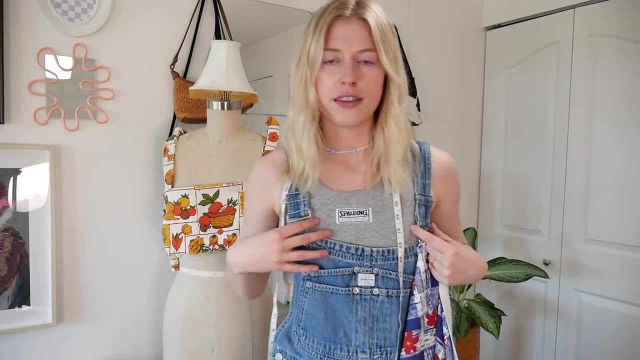 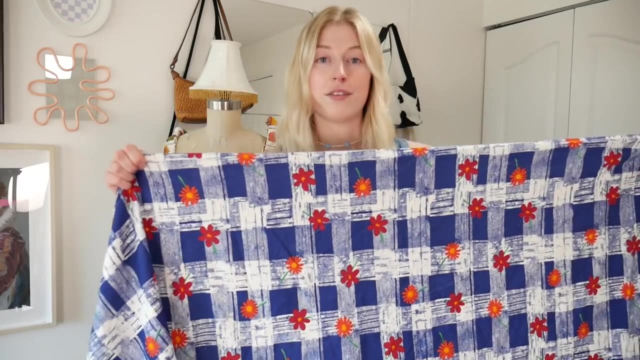 So mine's like third, I think. so I measured mine on top of my clothes and I think it was about 35 inches, So I'm going to double that. So I need 70.. I need 70 inches wide of fabric. 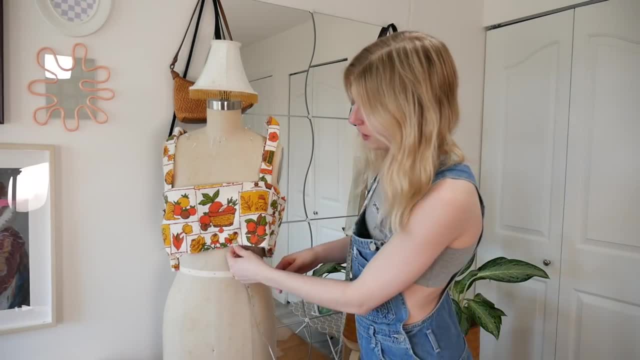 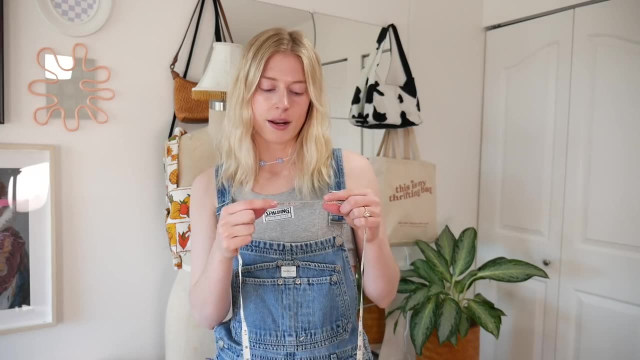 Then the next measurement you need is you need to measure from here, where you measure the top to the length you want. So mine is about 21 inches, and then I'm going to go ahead and I'm going to add two more inches for the seam allowance. 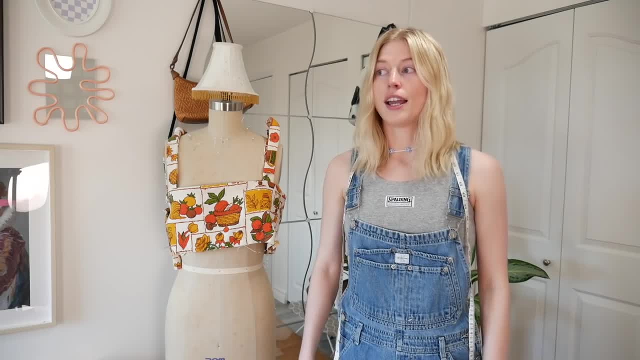 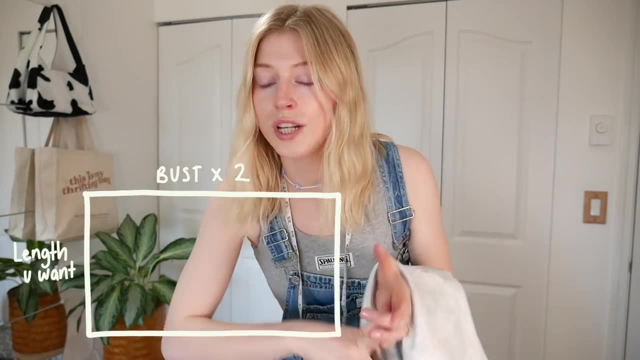 I need to cut out a rectangle that is 70 by 23.. Okay, before I cut it out, I just want to, you know, do a little recap. for the width of the fabric, You need two times your bust. for the length, It's just the desired length you want for your skirt. good, 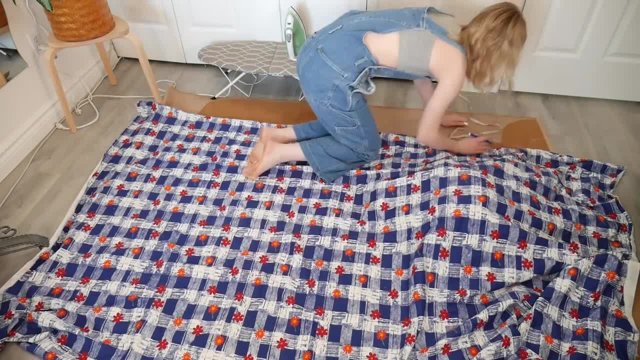 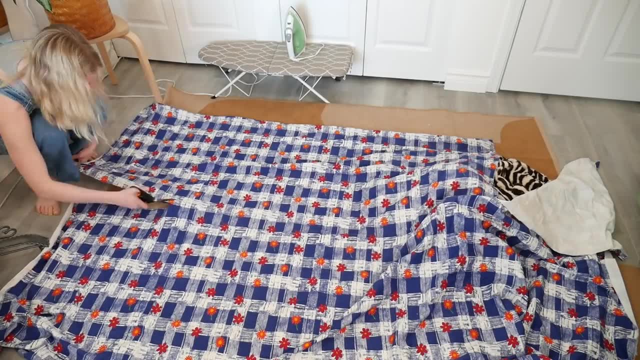 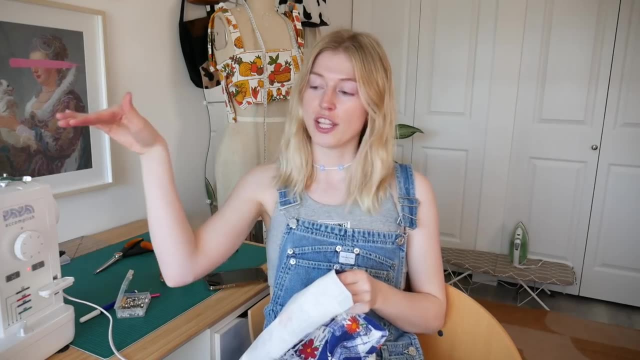 I'm going to cut mine out now. So now I'm going to do my gather stitch. which I like to do is I just like to do a one stitch, with no backstitch at the beginning or the end, and I like to do On four or five for the stitch length and then at the end. 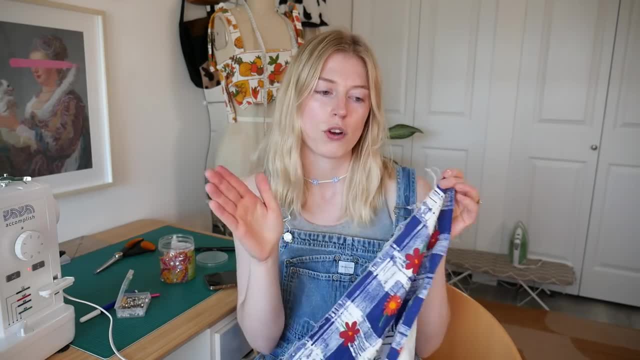 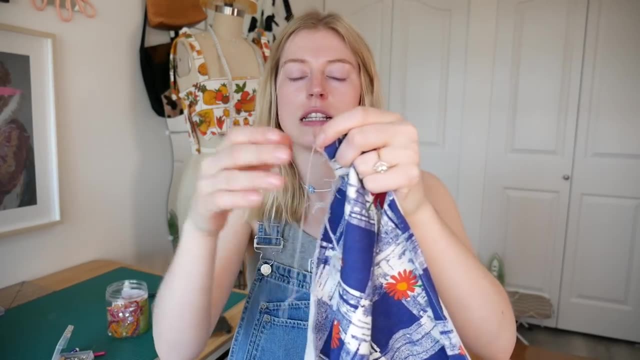 I like to just tighten it and gather it that way, so I can decide where I want the gathers. So once you have that stitch along the top, you can go ahead and you can take the string because you want to leave it a little bit longer and you 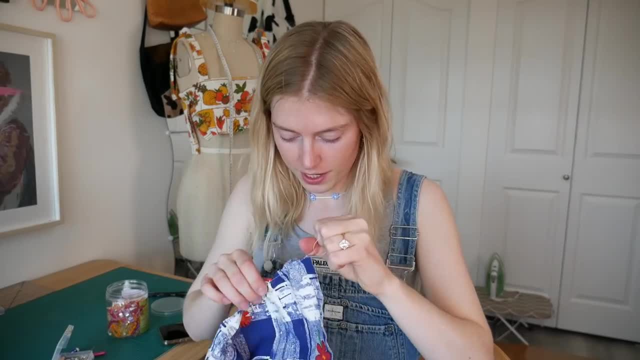 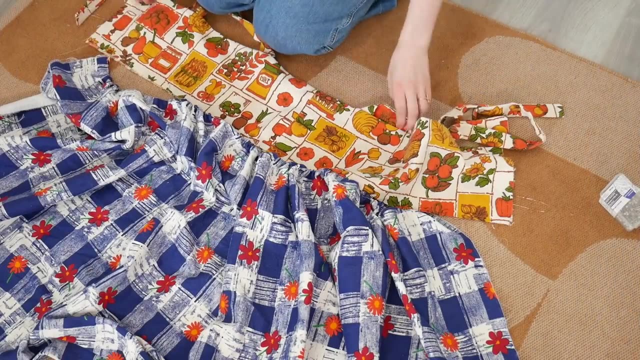 can just pull the top string and you'll start to gather like that. I just got to keep doing this gently because you don't want to break the thread, Otherwise you're going to have to do that all over again and stitch it. and then, once I was done gathering, I attached it to the front. 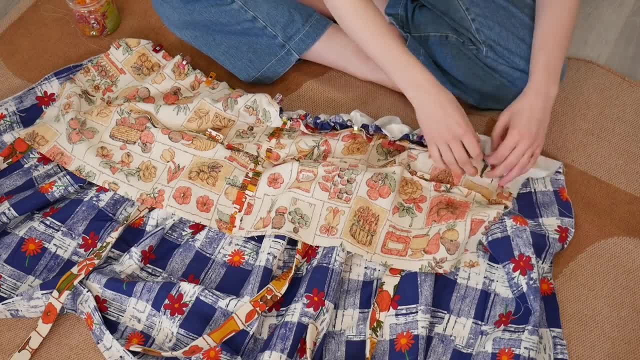 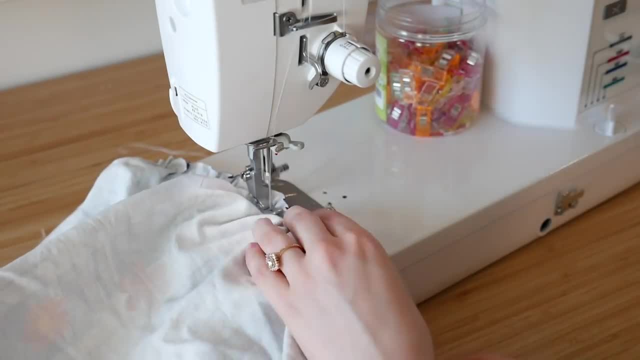 Of the top there and I just pinned it together, right sides together for the whole width of width, Yeah, width of the dress. and then, once I did that, I took it to my sewing machine and I just did a straight stitch, even though it's kind of weird. 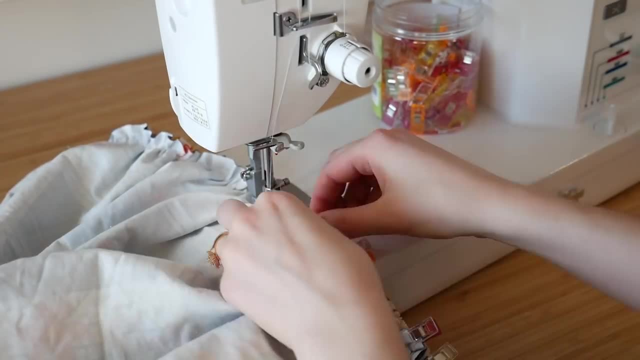 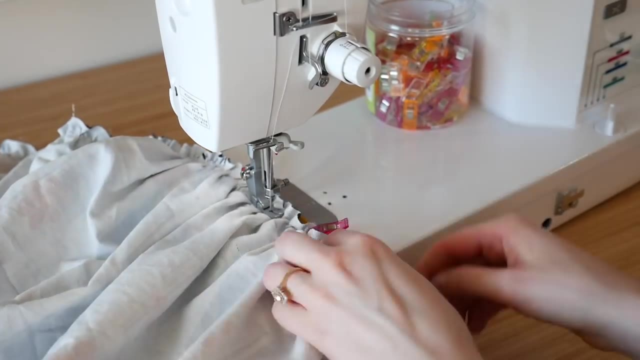 I always find it so weird when I'm straight stitching with this gather here. It just feels like you're not supposed to because there's so many lumps and I'm so used to sewing- you know a flat piece of fabric- So it's a little weird, but trust me. 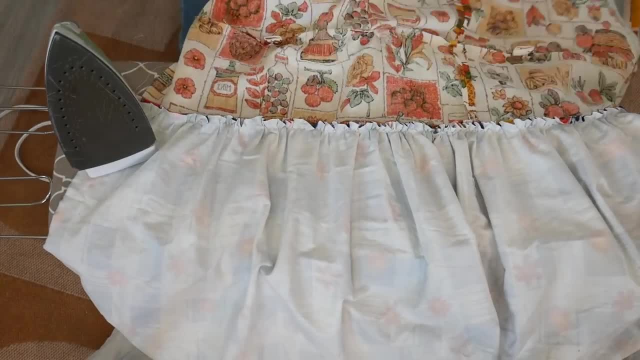 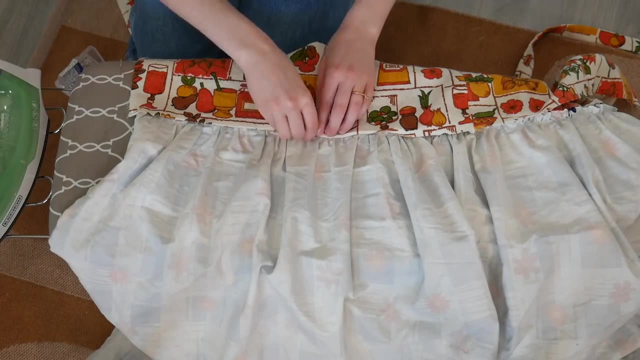 This is what you're supposed to do. after that, I took it to my iron and iron the seam Upwards towards the top of the dress, and then I took the lining of the dress, I folded the edge inwards- So you're not seeing any seam or any raw edge, and then I just ironed it. 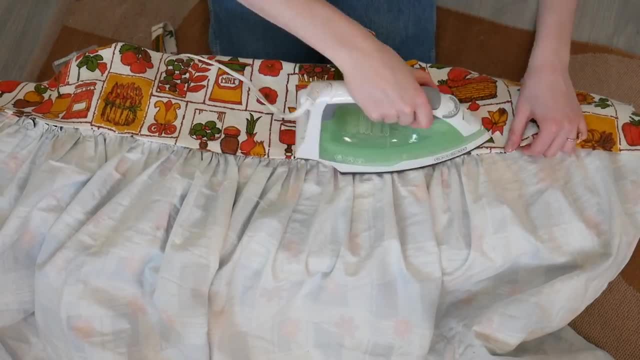 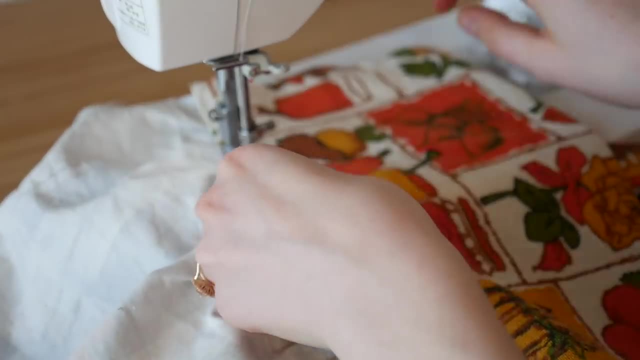 like that for the whole dress, and then I also put some pins in there because we are going to be sewing it down, So we actually have a nice finish inside the dress. So this part is a little tricky because you can't see your seam allowance. 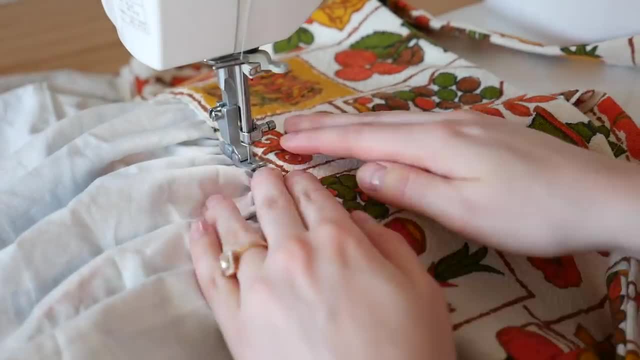 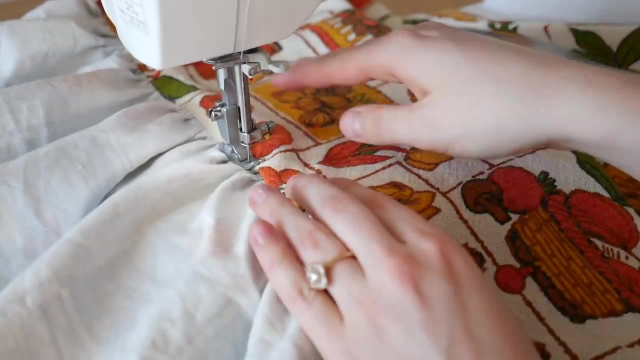 line. So what I like to do is I like to line up the edge of the fabric Work there to the edge of the presser foot on the left hand side and just kind of focus on that to sew a straight line. and then that's what I 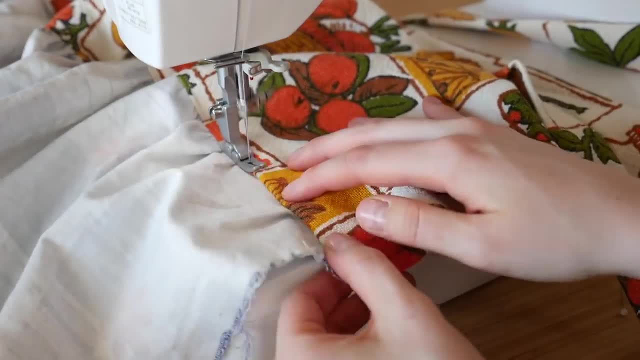 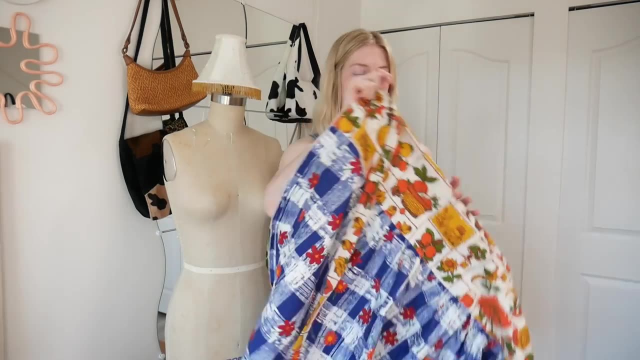 do for kind of pieces like this, where you can't see a seam allowance line. So here's my dress, Not sure how I feel about it, but we'll judge it at the end. Anyways, the next thing we're going to do is we are going to put the 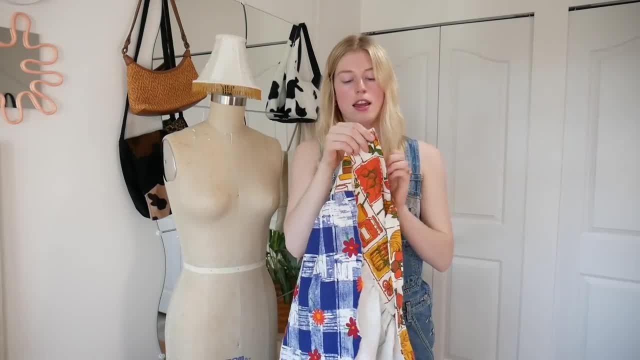 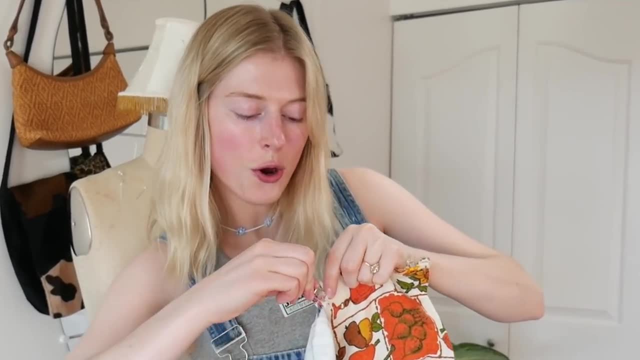 right sides together and we're going to take the two ends and we're just going to pin them all the way down The whole dress. It looks like this and once you have them pinned together like this, we're just going to do a straight stitch again. 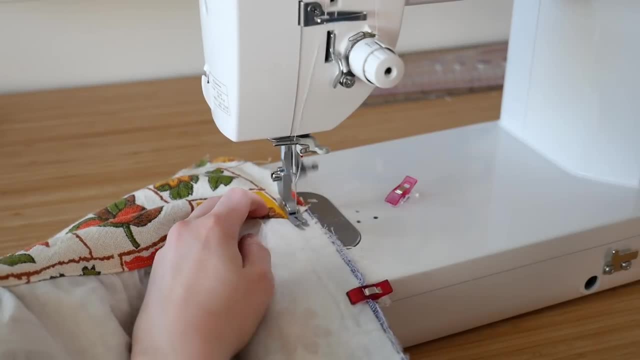 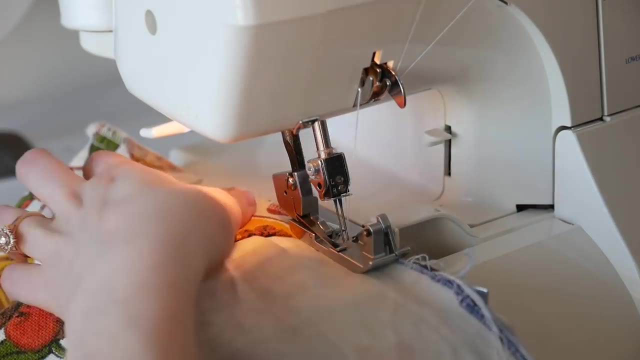 So I started off by doing a straight stitch with my sewing machine, But then after that I realized, hey, you probably should finish the seams off, So I took it to my serger and I just serged the edges. but most of you probably don't have a serger, so I would just zigzag the edges so it doesn't. 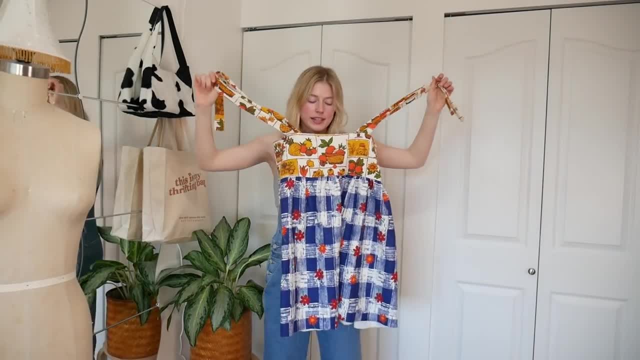 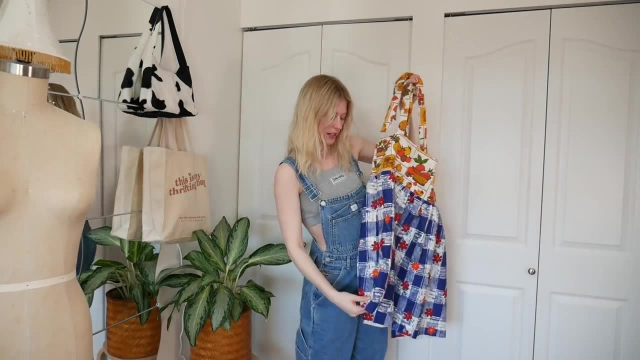 fray. And the final step to finish this Magnificent dress is: we need to hem it. We need to hem it. So I'm going to jump on my iron and I'm going to show you guys how you can roll it, So you guys can just jump in the sewing machine and just sew it one. 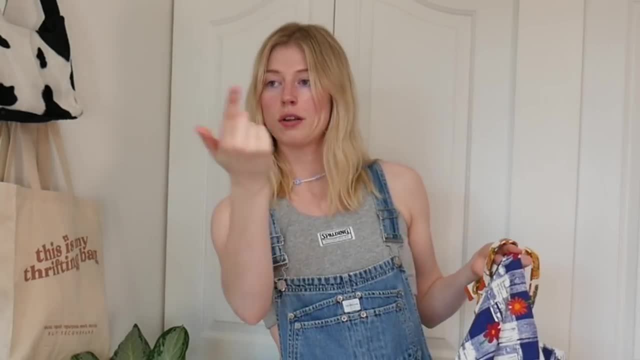 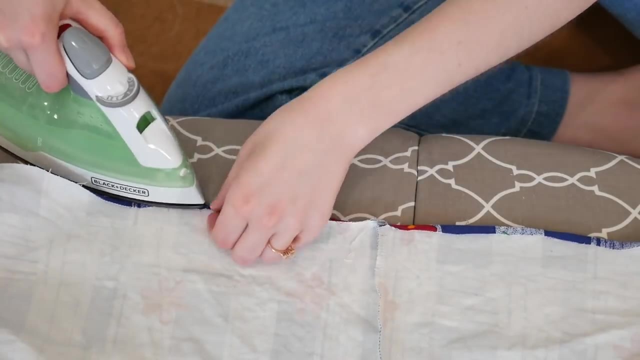 stitch, or one stitch around the bottom one time and then we're done the dress. So what I like to do for hemming is I fold it over just a little bit, like a quarter inch, half inch, all the way around the whole bottom of the dress or whatever. 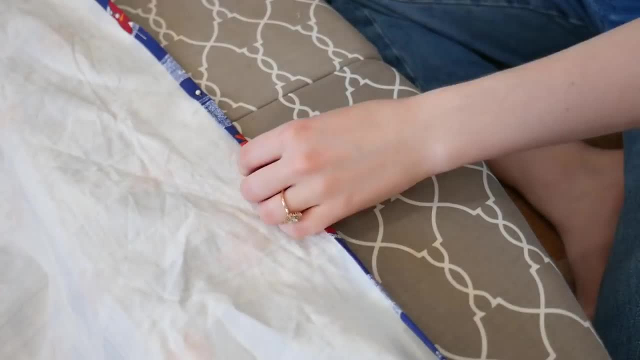 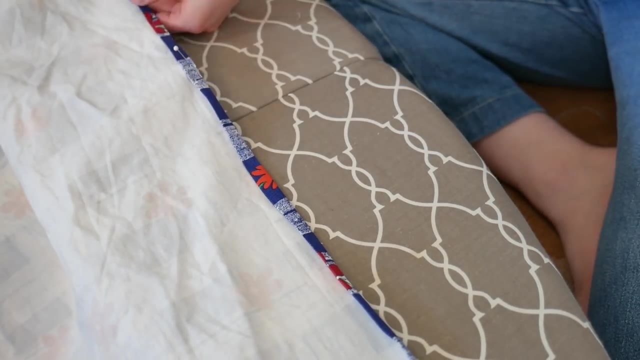 You're hemming, and I do that until I do the whole bottom. after that I go ahead and I fold it again once over, and then I also add the pins of the stage So it keeps it nice and secure. so we can go ahead and sew it after. so I 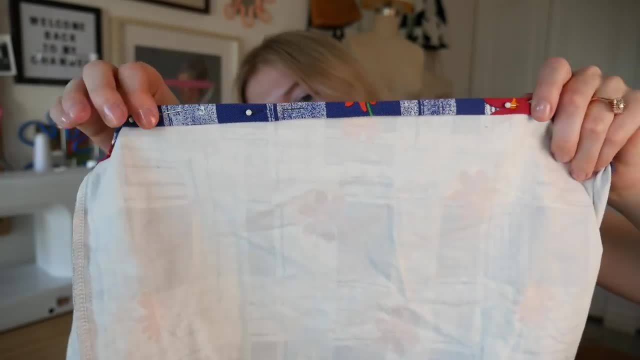 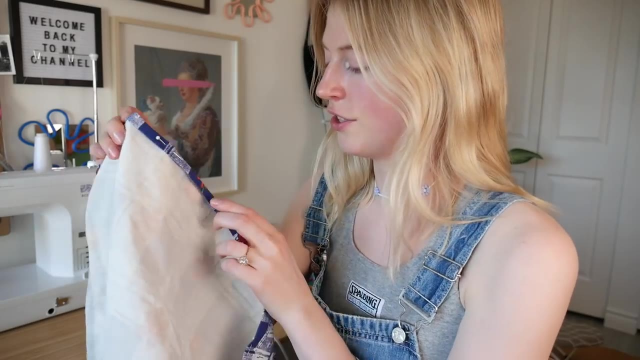 have it all ironed, I have it all pins, So it's nice and pretty the edge. So all they do is just do a straight stitch. I like to do a straight stitch really close to the edge here and I like to sew with this facing upwards, not this side, the wrong. 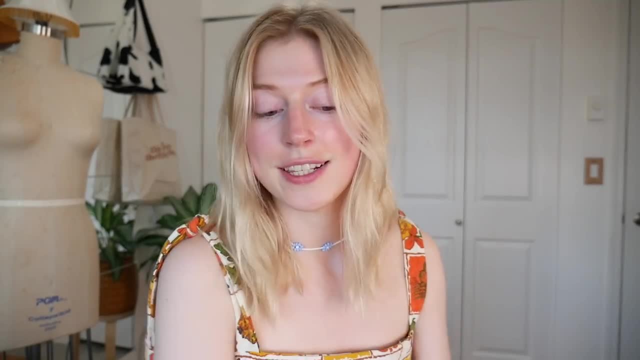 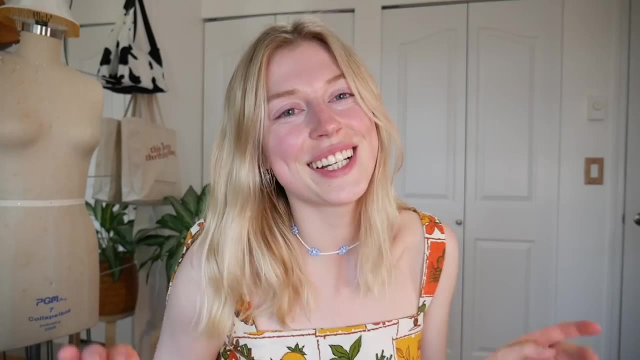 Side. So I am officially done the dress. I have it on, as you guys can see, but not fully. I'm going to show you second. but I did want to have a little disclaimer because it is a little out there, this dress, but I kind of dig it. 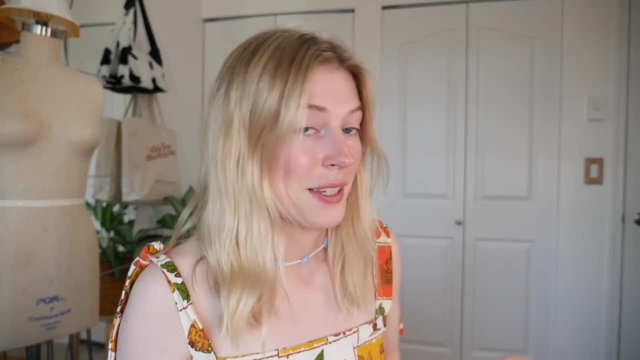 It's my cup of tea. It's not everyone's cup of tea, but it's my cup of tea, So that's all that really matters. So I'm going to show you guys the dress. I am super happy with it. I am thrilled.